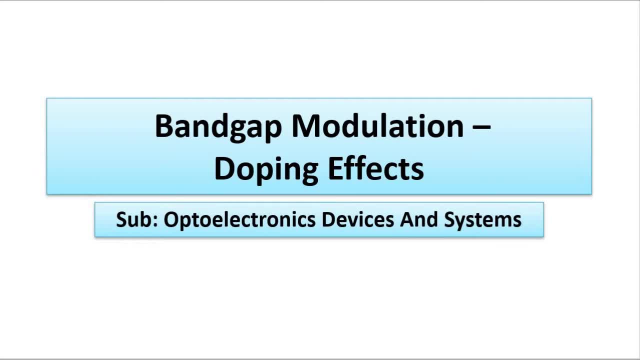 frequency or wavelength range of operation of, depending on our requirement. So in the previous video we discussed the compound semiconductors or alloy semiconductors method of band gap modulation. So in this video we are going to discuss about the doping method, the extrinsic semiconductor method or doping method, How we can use that to adjust the band gap. 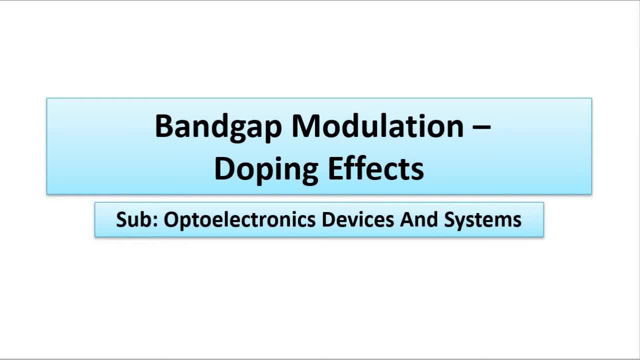 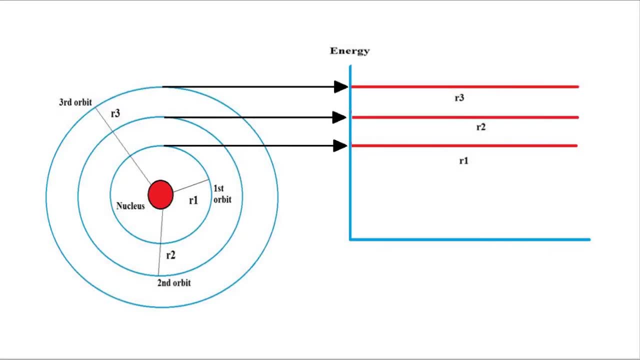 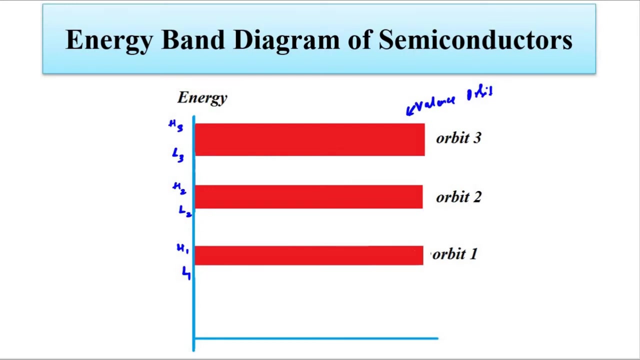 value, the forbidden energy gap value. So before that, just quickly, we will discuss that. we know that each orbit of the semiconductor atom, the electrons present in it, they have a fixed energy value. For isolated, single values, for multiple atoms, we have a range of values, with the outermost orbit having the highest energy value, which is the valence band, the energy corresponding. 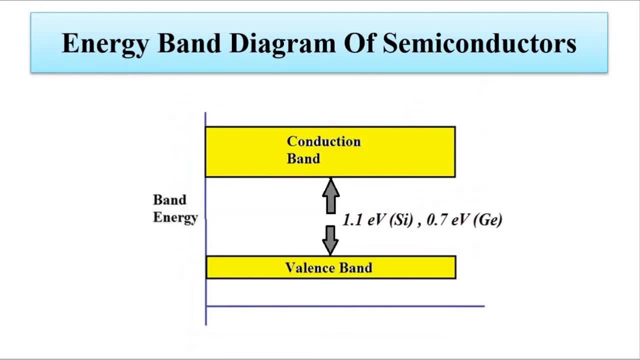 to the valence orbit And the difference between the valence band and the range of energies which is possessed by the free electrons, that is, the conduction band. that difference is called as the forbidden energy gap. So how electrons they move to the conduction band? One principle is that the electrons in the 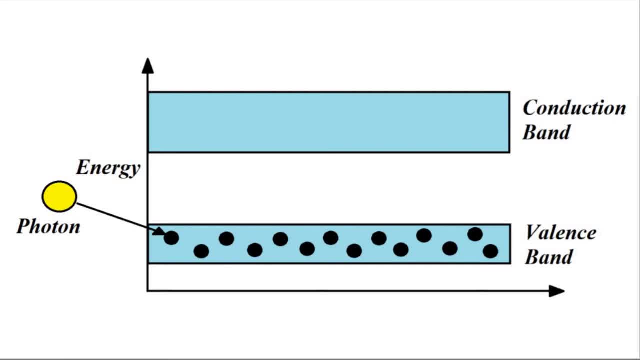 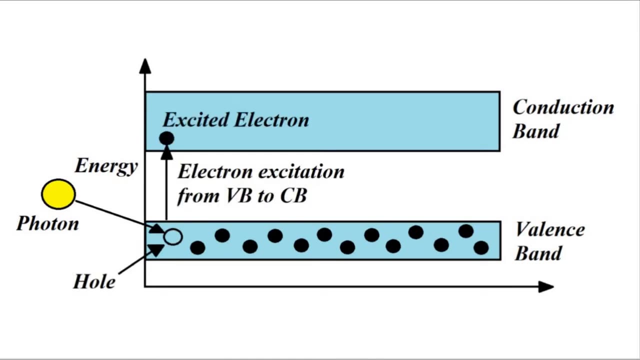 valence band. they absorb energy from light photons. I am talking from a optoelectronics point of view. When light falls on the material, the electrons in the valence band, they absorb a photon. Then they get excited to the conduction band, leaving behind a vacant electronic side hole, The excited electron. after a certain fixed period of time, which is the time period in the excited state, which is of the order of nanoseconds. 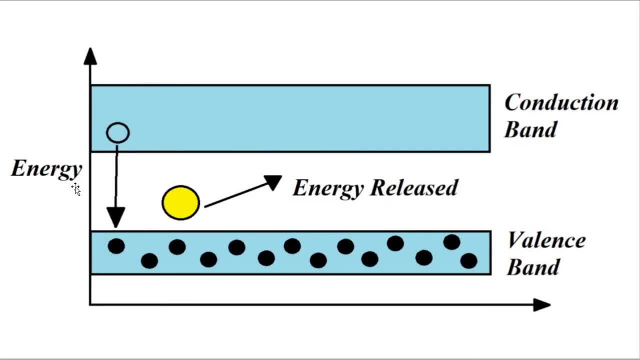 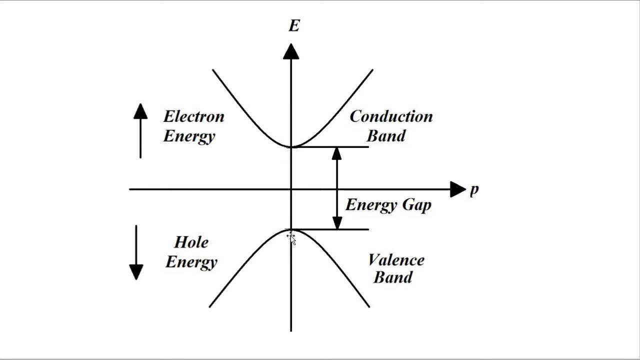 it drops down to the valence band again with the release of the photon which it absorbed initially. This is the basic principle And mostly. this transition of electron from valence band to conduction band is suitable for direct band gap semiconductors where the conduction band minima and the valence band maxima they occur at the same momentum value or same wave vector value. 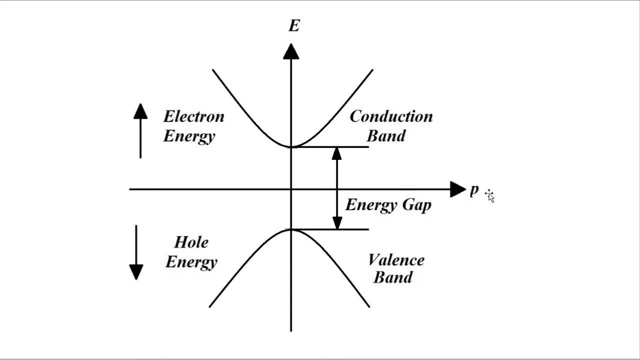 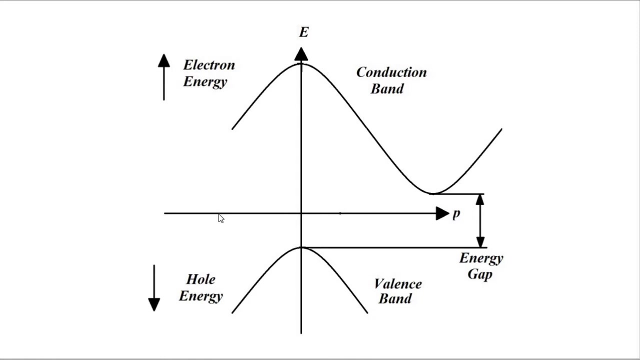 We have already discussed about energy momentum relationship, So this transition is very favorable. when the conduction band minima and the conduction band maxima. they have the same momentum value, This transition is smooth. Whereas for indirect band gap semiconductors, where they occur, the conduction band minima and valence band maxima occur at different momentum values. this transition is smooth. 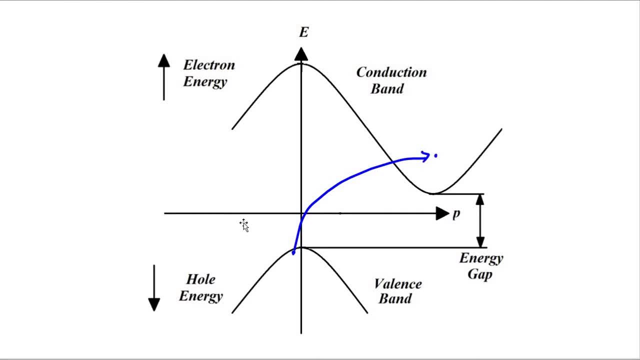 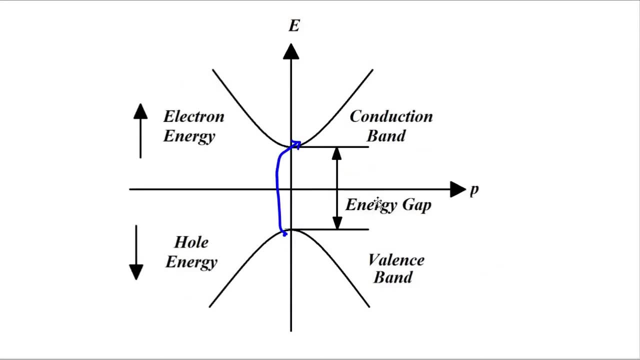 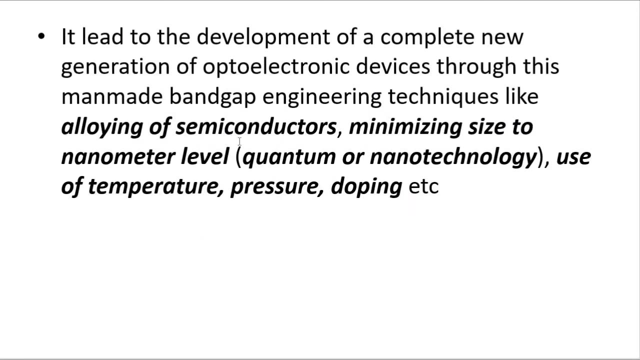 Not very easy. So, band gap modulation, adjustment of this forbidden energy gap, this energy gap modulation, or change. it can happen through different ways. One method we have already discussed, which is the alloy semiconductors or compound semiconductors method. 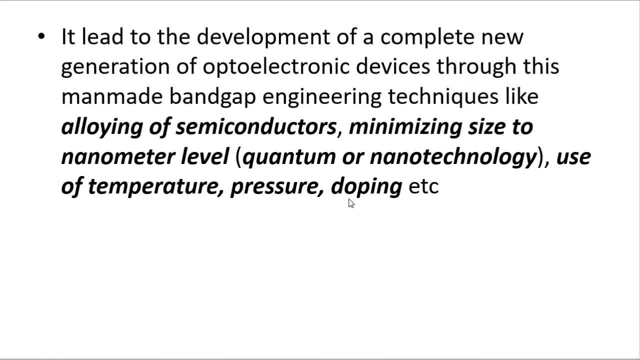 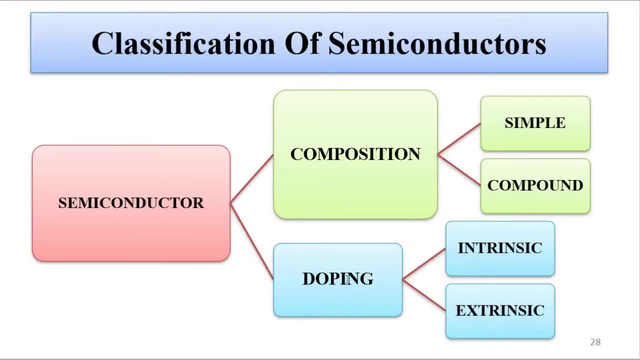 In this video we are going to discuss the doping method, doping. we know that the classification of semiconductors on the basis of doping is intrinsic and extrinsic. intrinsic semiconductor and extrinsic semiconductor. so this extrinsic semiconductor is called as a doped semiconductor. doping is the process of addition of foreign. 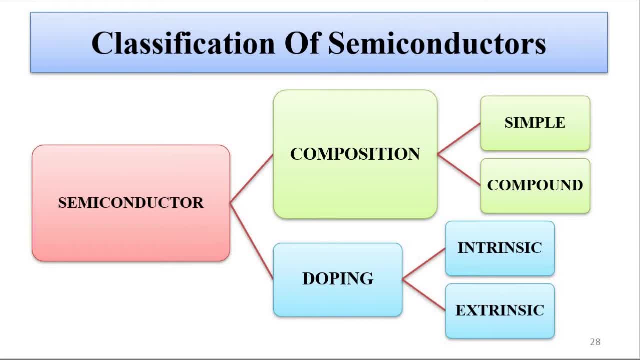 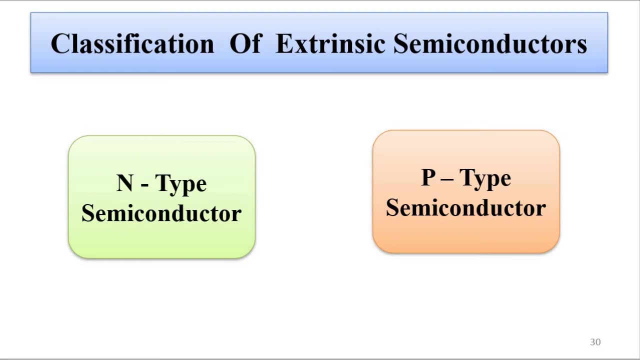 substances or impurities- pentavalent or trivalent impurities- to enhance the conductivity of the semiconductors by adjusting the band gap, energy value. so extrinsic semiconductors or doped semiconductors. they are of two types: n type and p type. n type semiconductors are those in which 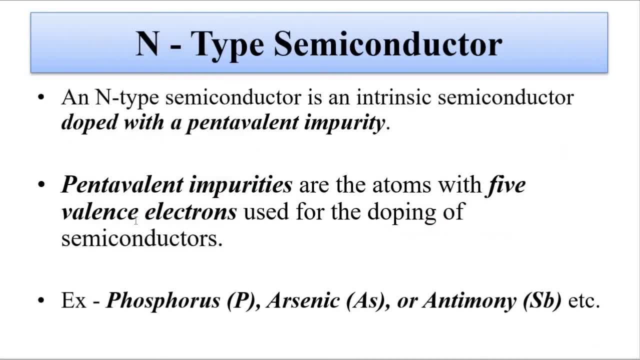 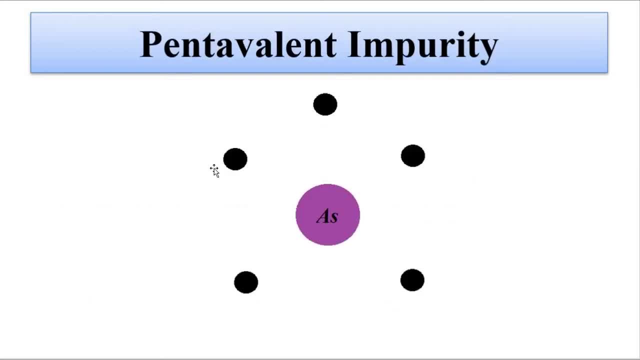 the intrinsic semiconductors are doped with pentavalent impurities. pentavalent impurities means impurity with five valence electrons, five electrons in the outermost orbit. for example, arsenic, intrinsic silicon or any other semiconductor is generally has four electrons in the outer orbit. so when these two combine, what happens? 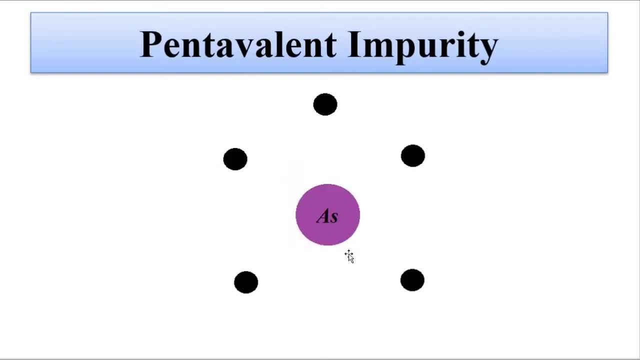 four out of the five outermost electrons of arsenic. they enter into covalent bond with each of the four outermost electrons elements of silicon. okay, this four covalent bonds are formed. so four out of four outermost electron electrons of silicon are exhausted, but one electron of arsenic is left behind. 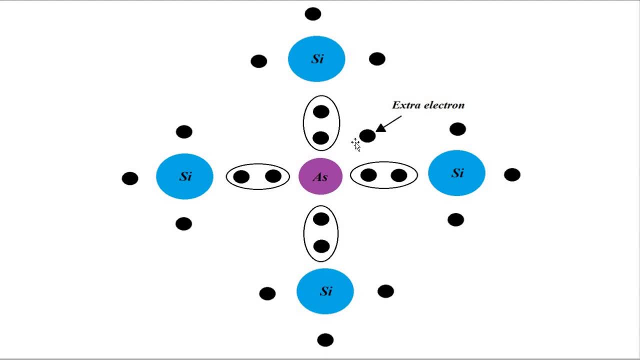 okay, this one extra electron from pentavalent impurity, arsenic. this extra electron is responsible for conductivity and it goes to the conduction band. so here the majority charge carriers are electrons negative charge. that's why it is called as n type semiconductor. okay. 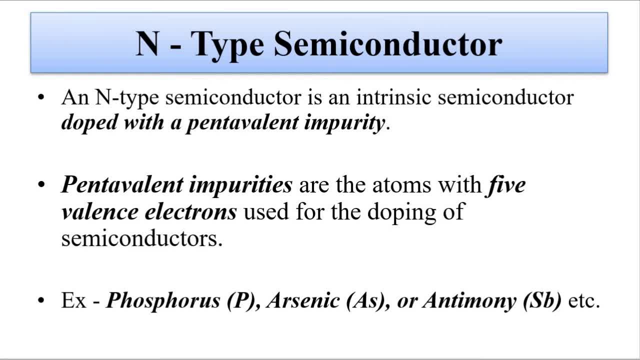 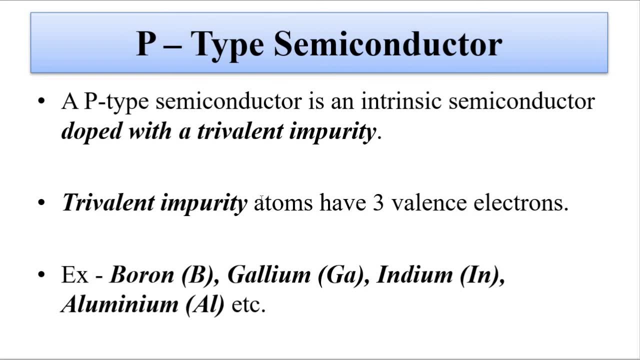 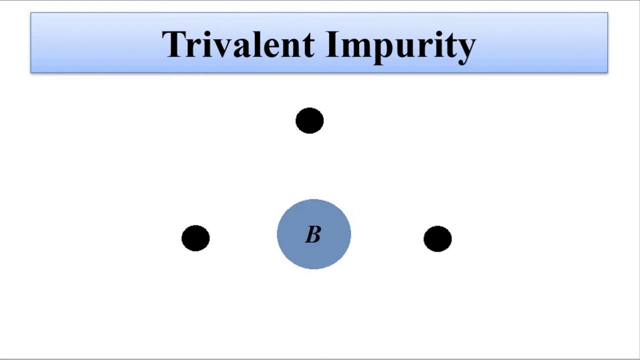 So another process is the p type semiconductor, where silicon is doped, or silicon and any other semiconductor is doped with trivalent impurity. so what is a trivalent impurity? trivalent impurity Is one one in the valence band or outermost band, okay, this, for example boron. So here, when the trivalent 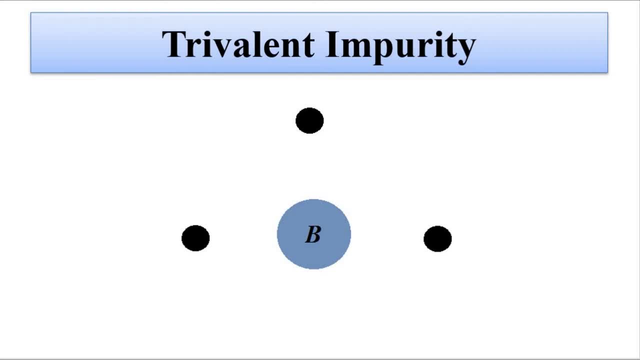 impurity, combines with silicon or any other. not silicon, because silicon is not used in optoelectronic purposes, because it is indirect band gap or any other semiconductor electron, a semiconductor element, because they all have four outermost electrons- what happens is that three out of the four semiconductor atoms- for here I am just using silicon as an example- 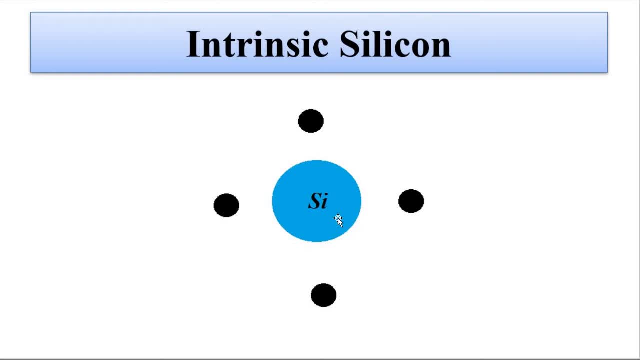 do not take it as a, you know, as a constant thing here. just I am giving you example of p type and n type semiconductor formation. Silicon is not used for optoelectronic purposes because it is indirect band gap, Band gap semiconductors. okay, it is indirect band gap semiconductor which is not used for. 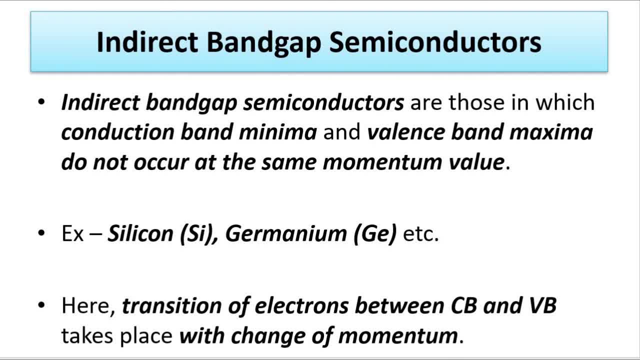 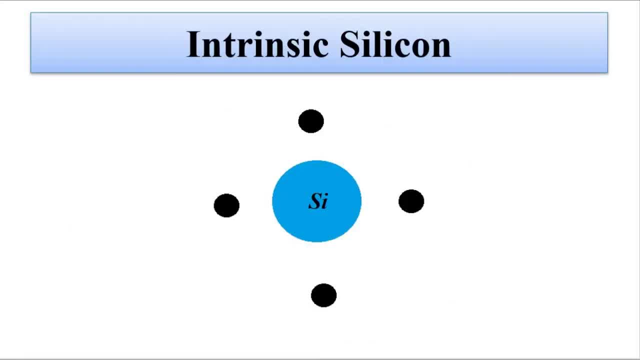 optoelectronic purposes only direct band gap semiconductors are used, compound semiconductors. So here I am just using silicon as an example. So here what happens? three out of the four valence electrons of silicon enter into covalent bond with three out of three of boron and 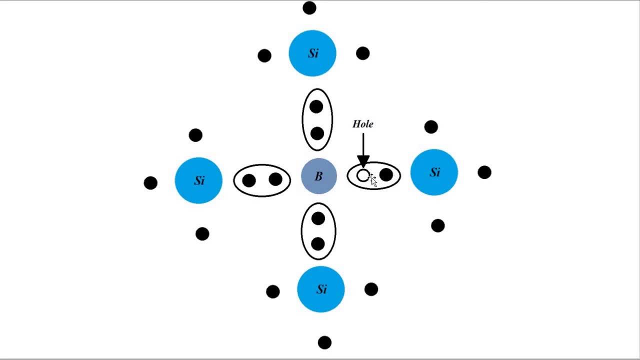 one such covalent bond formation with silicon atom. So what happens here? then you have a one demand. electron is theipse mystery. can cease it at noactus n t point c, that 0 pick n point d, p and is acting with the electron, no oppressed. 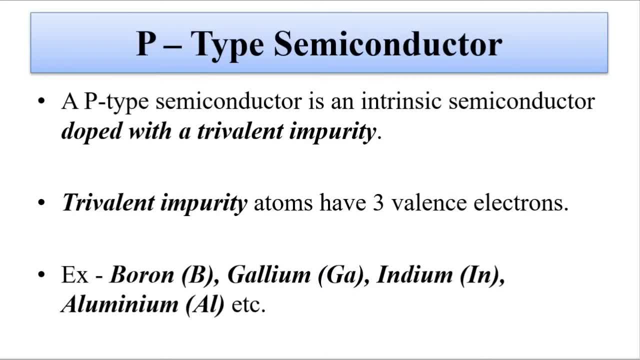 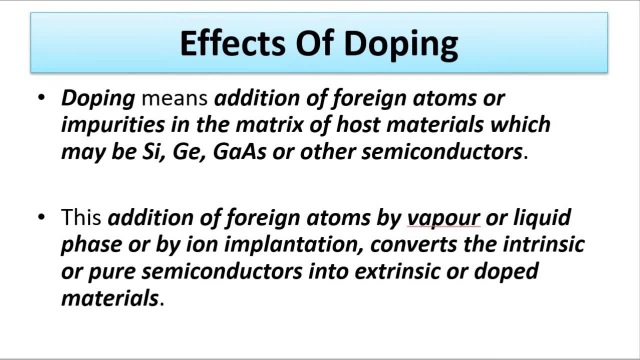 electromic bonded electron. So as you see, this electron, no oxidant. So what happens here to do with this conductor? So you called this modulate electron. if we say p, one allowed energy. So what happens? The addition of these foreign impurities, it leads to a large 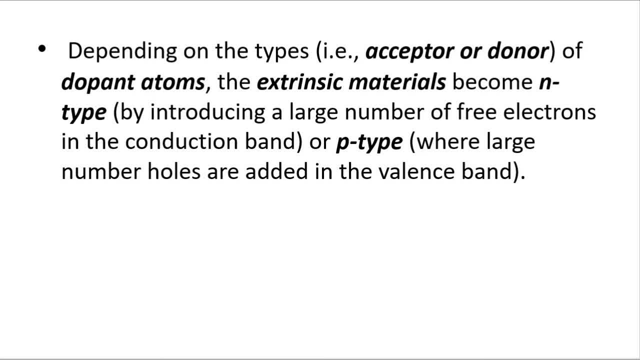 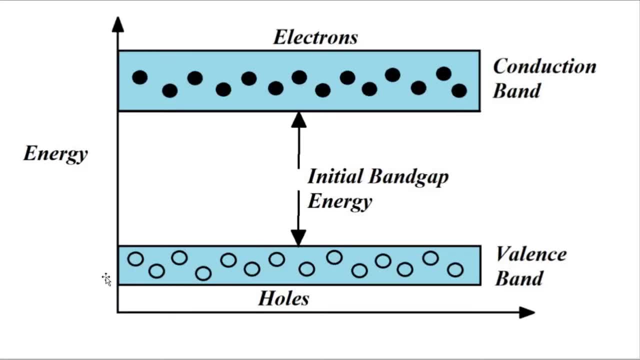 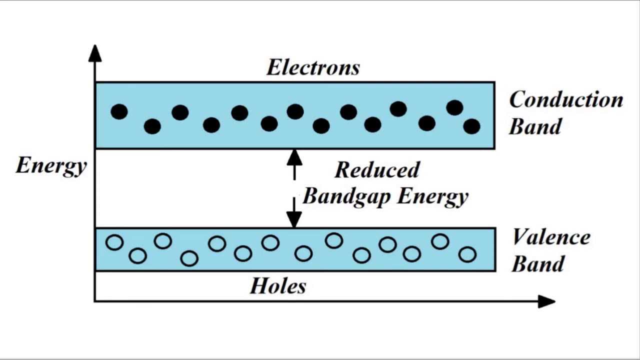 number of free electrons in the valence band, free electrons in the conduction band for n-type semiconductors or holes in the valence band for p-type semiconductors. So initially, if the initial band gap energy is high after doping, it gets lowered. It gets lowered Why? 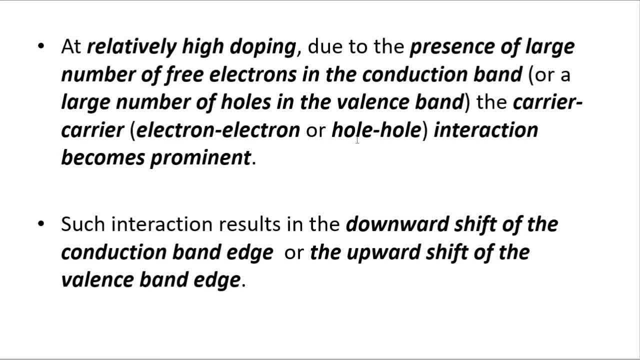 Because of the electron-electron or hole-hole interaction. It is electron-electron in case of n-type semiconductors because it is the majority charge carrier. In case of hole-hole, it is because of p-type extrinsic semiconductors. In n-type extrinsic semiconductors, electron-electron interaction. 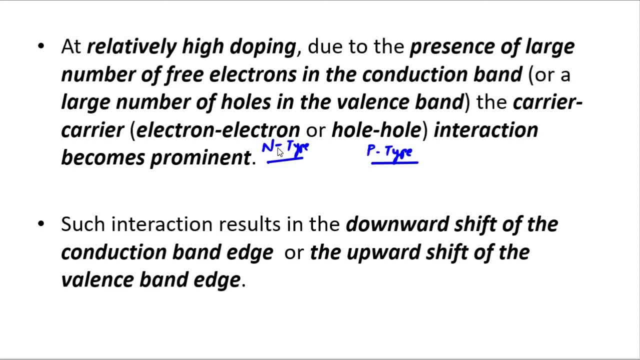 happens In p-type semiconductors. hole-hole interaction happens because in n-type electron is the majority charge carrier, In p-type hole is the majority charge carrier In the sky, whereas in Normal a compares u-texture Any d-comp. 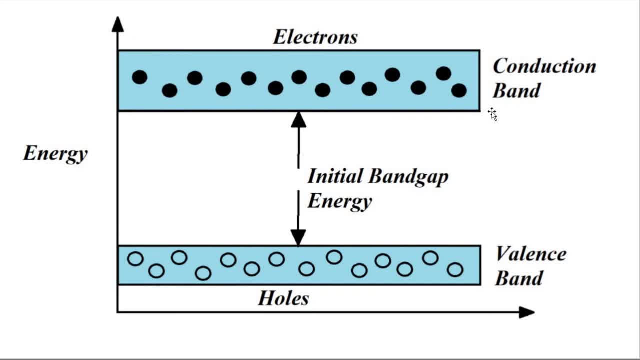 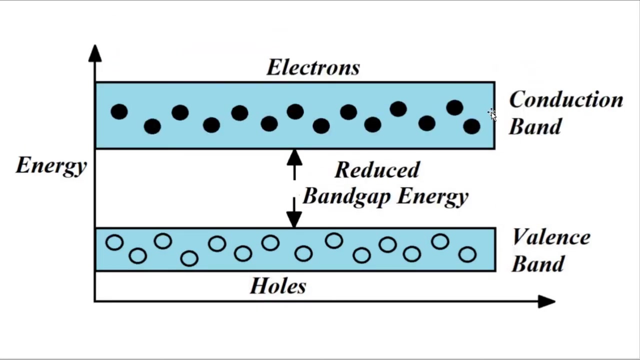 It will look a bit more like an elevation matrix. In that escalation matrix, the applied the Xy-Y-Zn-C, The teammate zone, constant, extended. the energy In answers you well, Are you OK? and taking, Of course, is shifted upwards or the conduction band goes downwards. in both the cases we have one result. 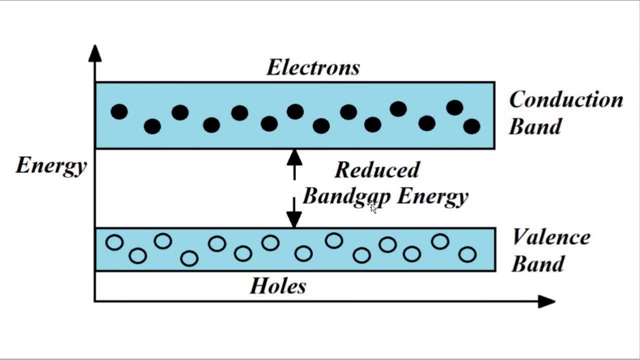 one common outcome, that is, the band gap energy. the difference between the conduction band and valence band will be lower. that is what we want, because the lower the band gap energy, the less the energy will be required for transition of electrons from valence band to conduction band. 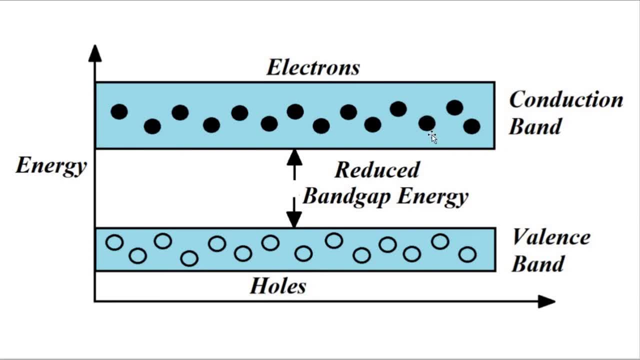 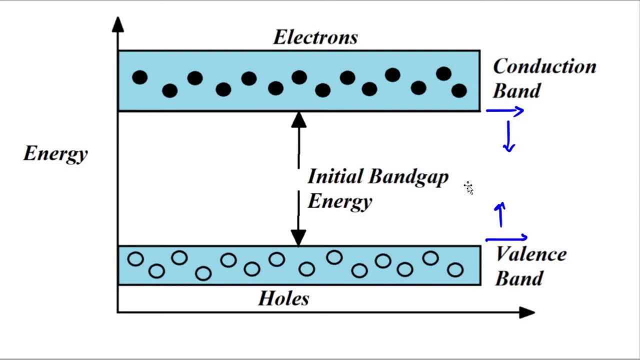 and the more the number of electrons in conduction band, the better the conductivity. okay, so we want one outcome: band gap energy to be reduced. whether it happens through conduction band going downwards or valence band going upwards, no matter, we want the band gap energy to be. 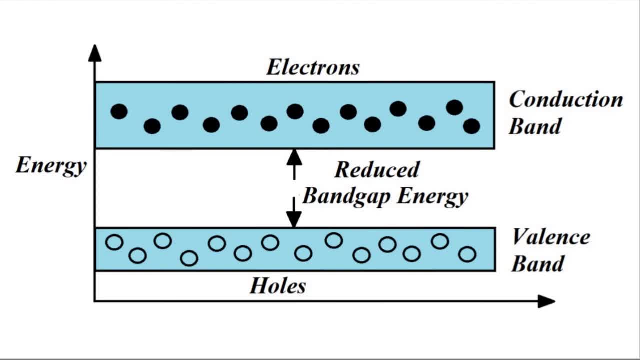 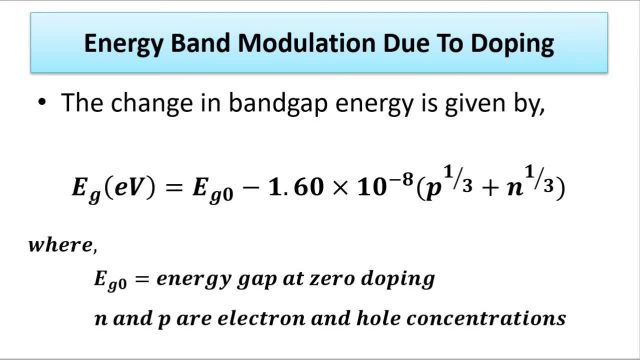 reduced. that is the outcome that we want and that is what happens here. so if we want to get a mathematical expression, the change in band gap energy is given as per this formula. okay, the band energy in terms of electron volt is equal to the band gap energy, the initial value at zero doping, when the semiconductor was in its pure 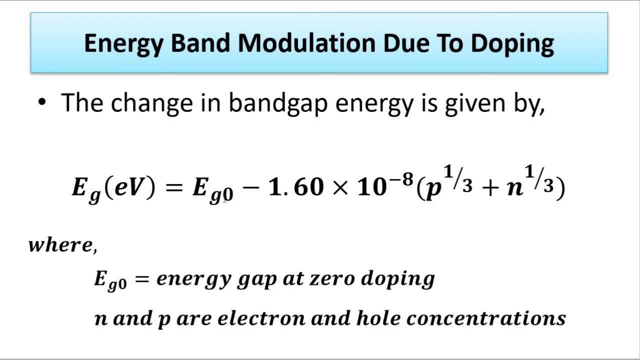 state intrinsic form. when no foreign substances, pentavalent, trivalent, whatever, when no such impurity is added, no doping happened. the band gap energy at that is called as eg0. and when doping happens, this, this factor comes into play. this value, one point six, zero, and return to power minus eight, p to the power one, by three plus n to the power one. 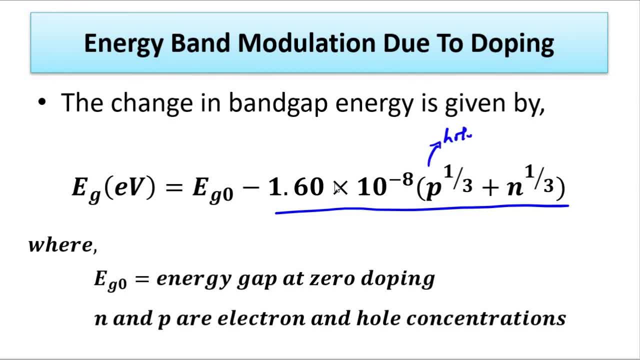 by three, where p is the whole concentration and n is the electron concentration. so always remember, in any situation there will always be the existence of electrons and holes. in n type also, holes are there, but they are minority charge carriers. semiconductors: there are electrons, but they are minority charge carriers. So always remember. 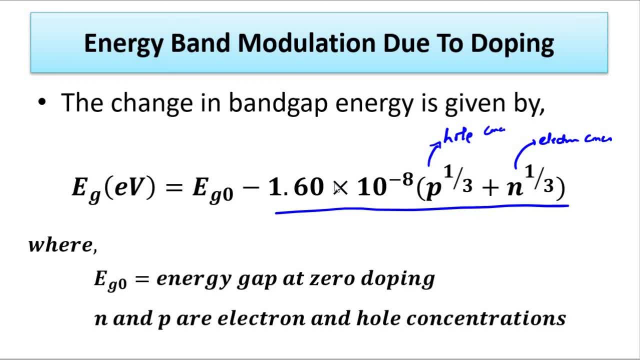 majority and minority charge carriers In n-type semiconductors. electrons are the majority charge carriers, holes are the minority charge carriers. Current conduction happens because of both contribution of both, but one is in majority, one other one is in minority. Similarly in p-type. 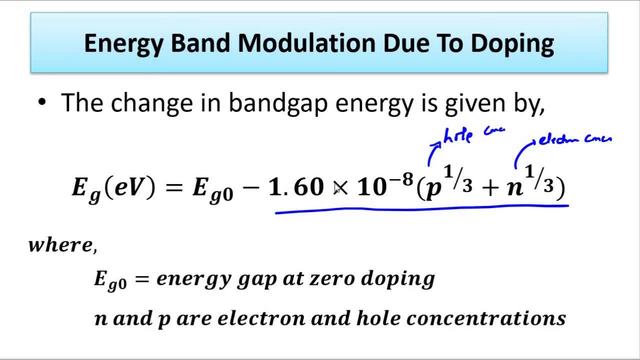 semiconductors. holes are the majority charge carriers, electrons are the minority charge carriers. So these two factors will always be there. One concentration will be high. the majority one will be high in concentration, the minority one will be lower in concentration.